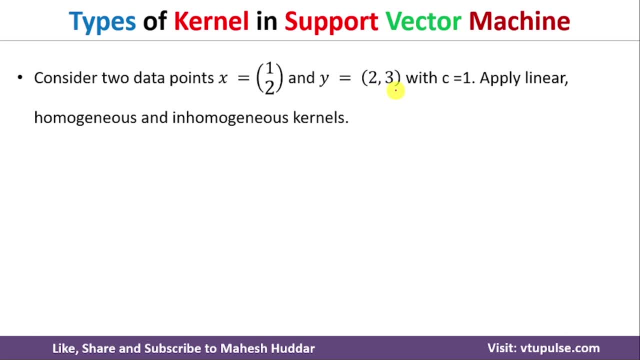 equivalent to 1, 2 and y is equivalent to 2,. 3 are the two data points, with c is equivalent to 1.. Now we will try to apply linear, homogeneous and inhomogeneous kernels over here. The kernel is given as k, xy is equivalent to x. transpose y raised to q If the value of q is. 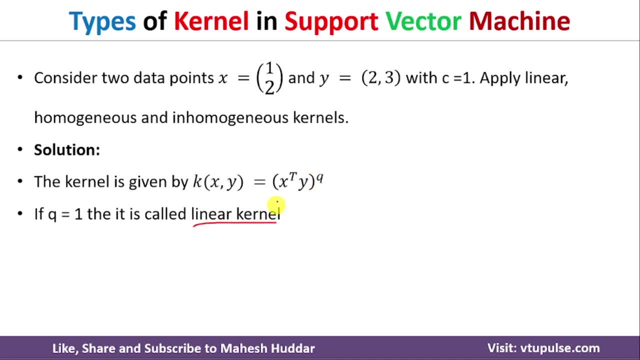 equivalent to 1,, then it is called as the linear kernel. If the value of q is equivalent to 1, then it is called as the linear kernel, And then we will put the values of x and y over here. So x is 1, 2 transpose 2, 3.. So now we need: 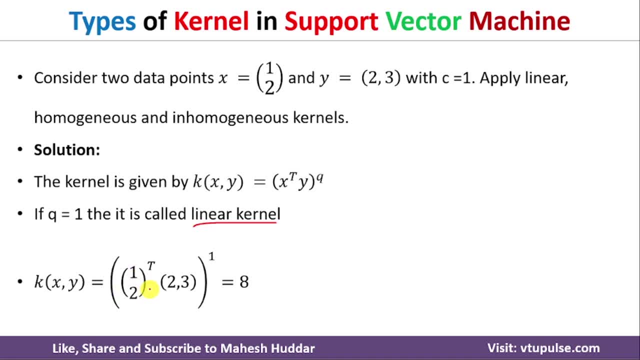 to take the transpose of 1, 2, that will this column will become a row here. So, and then we need to take the dot product, that is, 1, 2, dot 2, 3.. If you perform that particular thing, 1 into 2 plus. 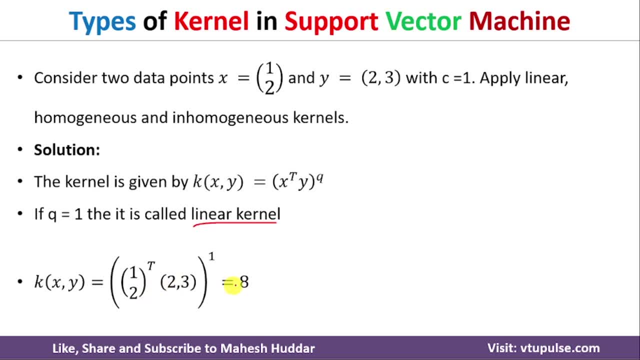 2 into 3, that is 6,. 6 plus 2 is equivalent to 8 over here. So the value of linear kernel is 8 for these two data points. in this case, If the value of q is equivalent to 2, then this is already calculated, which is equivalent to 8,. 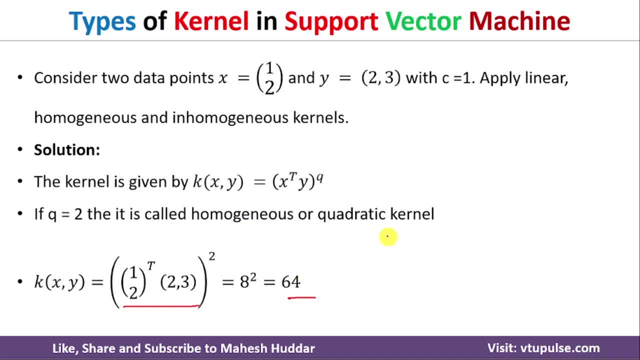 8 raised to 2, which is equivalent to 64.. For homogeneous kernel, the value of this particular data point will become 64 over here Homogeneous, or you can say that the quadratic kernel in this case, because the value of q we have selected as 2 in this particular case. Now I will consider. 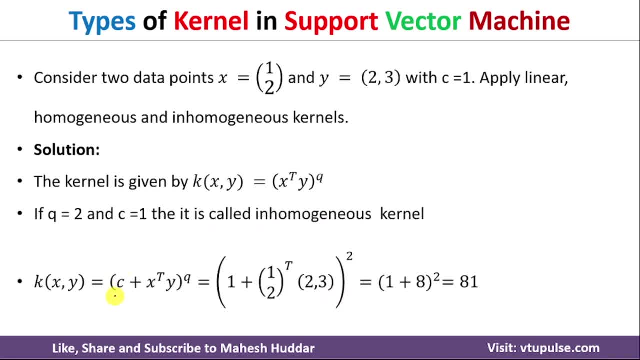 the inhomogeneous kernel where we will come across one more constant, that is c, c plus x. transpose y raised to q here. So c is 1, we have already calculated this one, that is 8, 8 plus 1 is equivalent to 9, 9 square is: 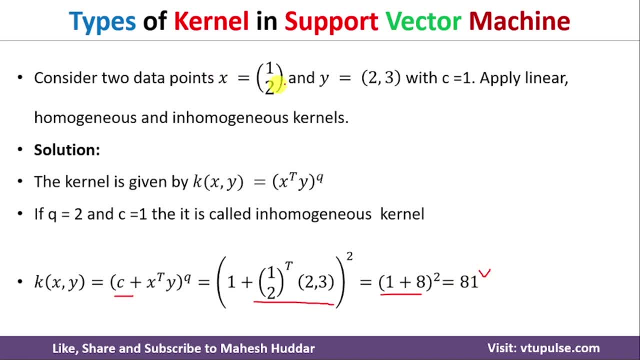 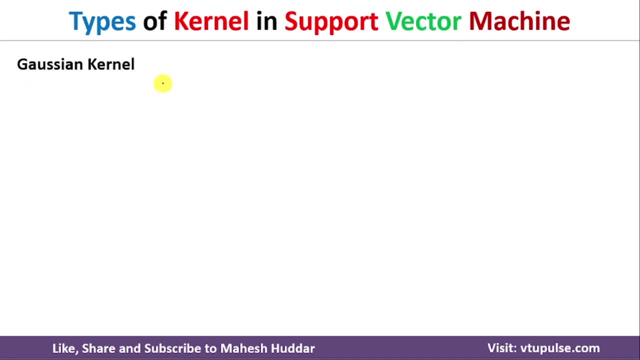 equivalent to 81 in this case, So 81 is the value of these two data points in inhomogeneous kernel. over here, Coming back to the next type of kernel that is known as Gaussian kernel. The Gaussian kernel is also known as a radial basis function or RBFs. They are extremely useful in 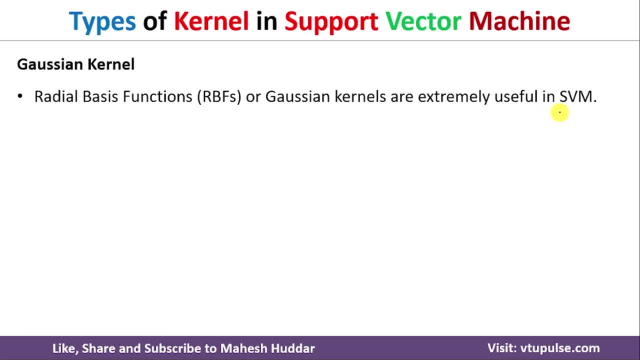 SVM because they perform very well on the given data set. So compared to other kernels, these kernel are extremely useful in SVM classifier over. here The performance of these kernel, that is, the Gaussian kernel, is very high. that is the reason they are extremely used in SVM classifier over. 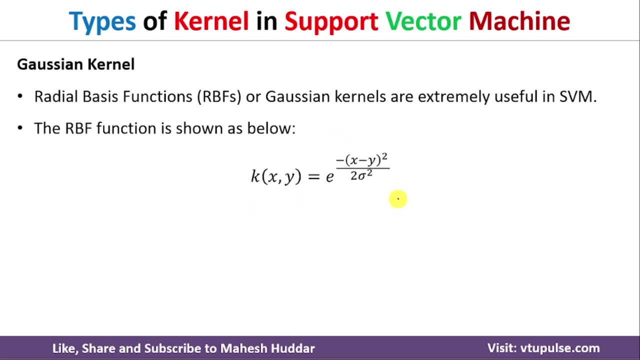 here The RBF function is given something like this: k, x, y is equivalent to e raised to minus x, minus y. bracket square divided by 2 delta square. Here x and y are the data points and delta is the constant over here. Now the value of y is very important in this particular case. If the 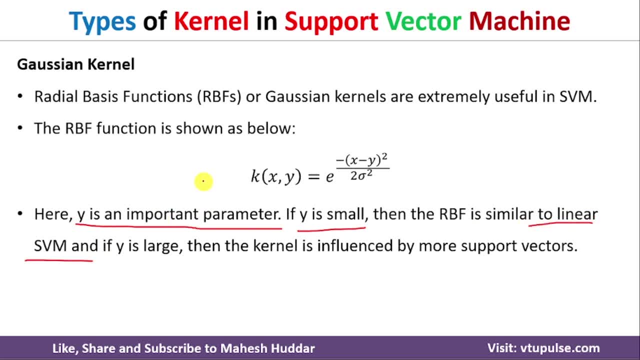 value is small. this will become a linear SVM, that is, the data point will be separated with the help of a straight line. If we select y, a large value, then we need to have more number of support vectors so that we can separate that particular data into two classes. over here, The RBF performs. 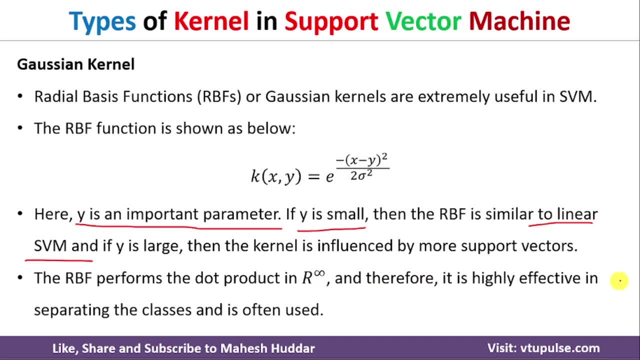 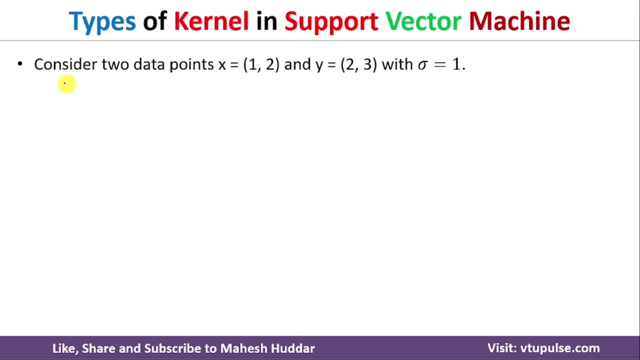 dot product in R infinity space. Because of this, they are highly effective as well as they are performance intensive, And that's the reason they are used extremely in the SVM classifier over here. Now we will consider one simple example to understand the Gaussian kernel. The first data point given to us is one, two, and second one is two, three. 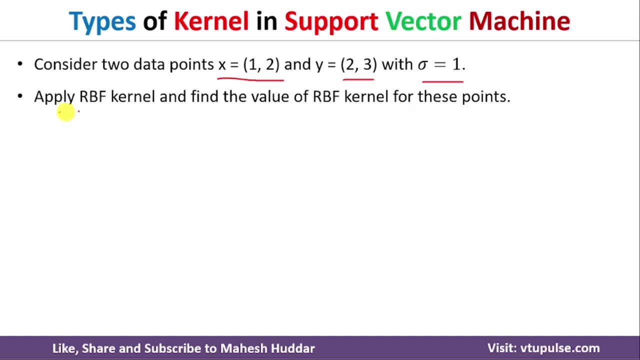 delta in this case is one over here. Now we will try to apply RBF and then we will try to get the value of this particular RBF value for these two data points over here. We already know how the RBF kernel looks like In this case. we need to calculate this: x minus y bracket square. 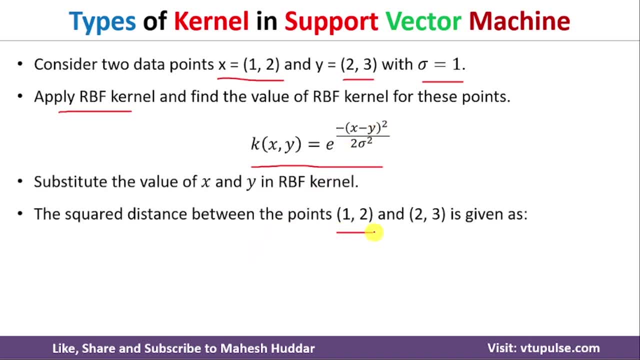 So first we will try to calculate that the first time x is two, one and y is two. second time x is two and y is equal to three over here. So one minus two bracket square and two minus three bracket square, which is equal to two over here. So this particular term, that is x minus y bracket square. 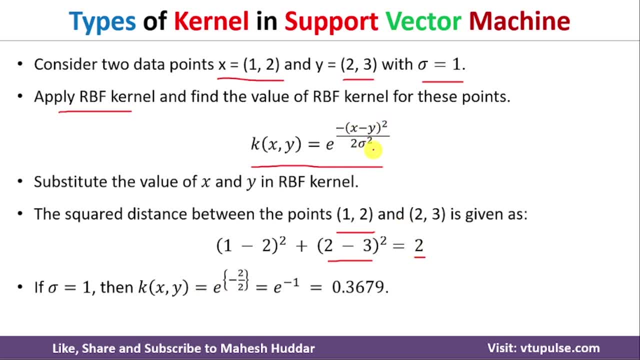 is equal to two. So e raised to minus two divided by two into delta square, that is nothing but one square. that is nothing but minus two divided by two over here, which is equal to e raised to minus one. If you solve this, you will get. 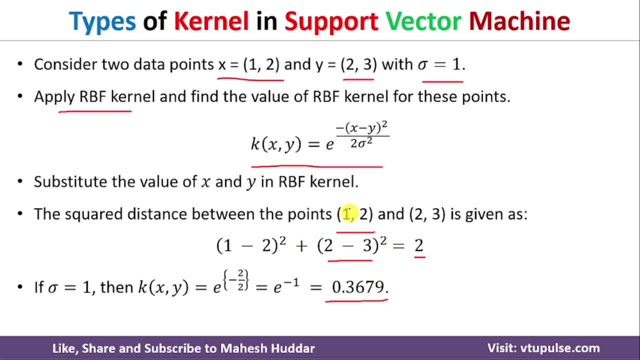 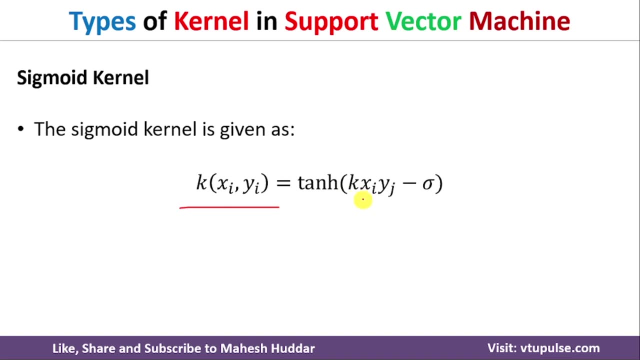 0.3679 in this case. So the value of RBF kernel is 0.3679 for these two data points, with the delta is equal to one in this particular case. The last type of kernel is the sigmoid kernel, which is given by k xi yi is equal to tan h, k xi, yj, minus delta in this case. So in this case,